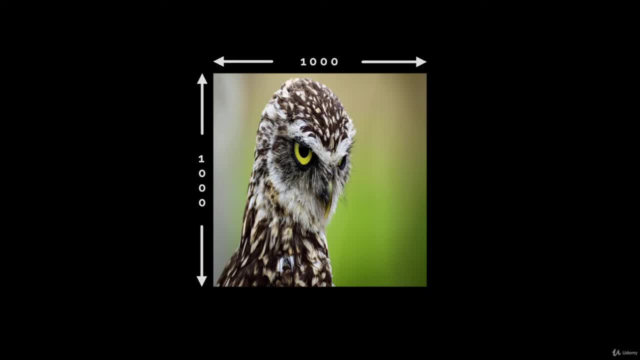 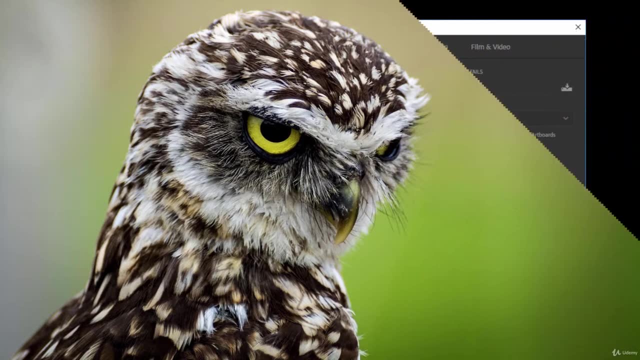 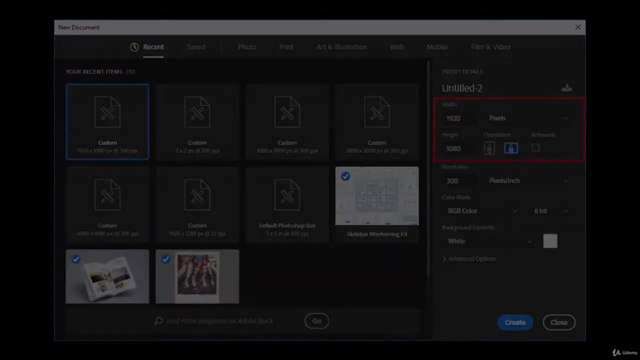 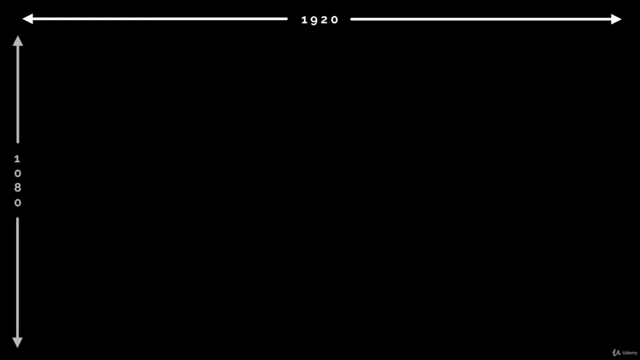 1000x1000 even looks smoother. Most high-definition devices like computer monitors and televisions nowadays are starting to be rated at 1920x1080 pixels. This means there are 1920 pixels horizontally, 1080 pixels vertically and a total of 2,073,700 pixels. 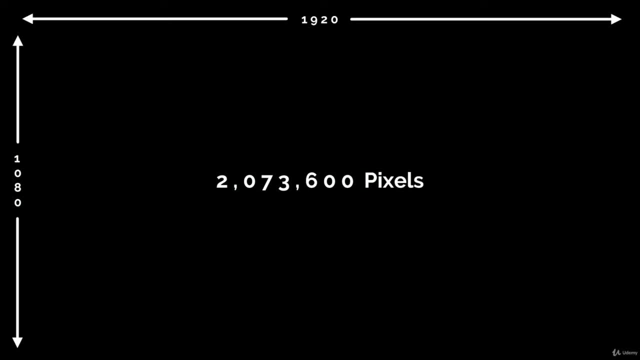 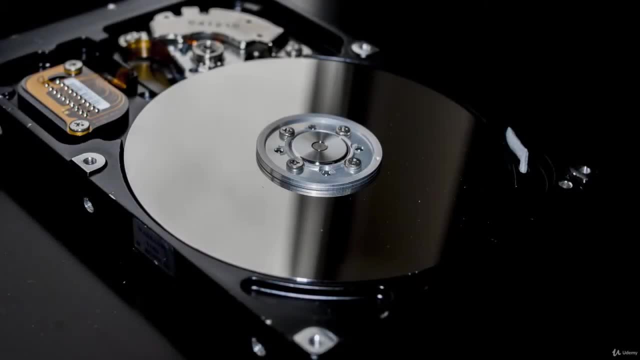 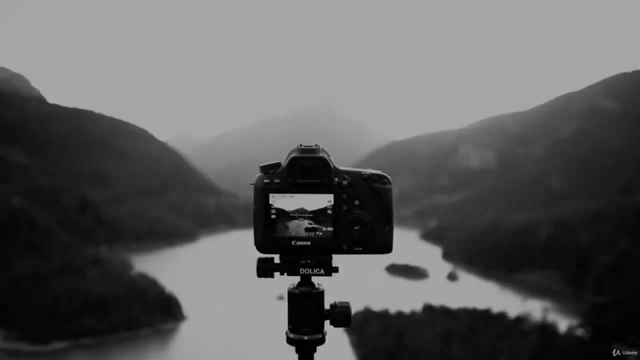 That gives a lot of pixel definition to our image and a much smoother look. It also creates a bigger file size, so it's important to know that the more pixels you begin adding, the more space it will take up on your computer. We are starting to venture into 2K and 4K resolutions, where the pixel dimensions are. 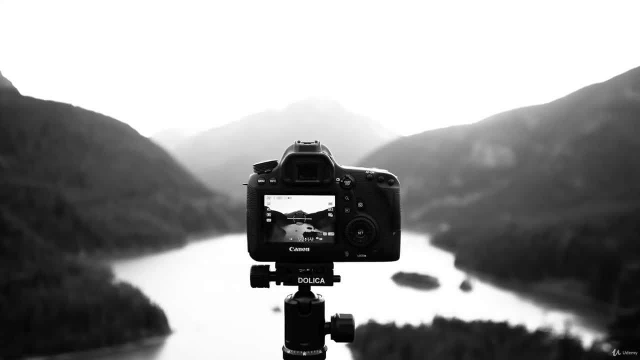 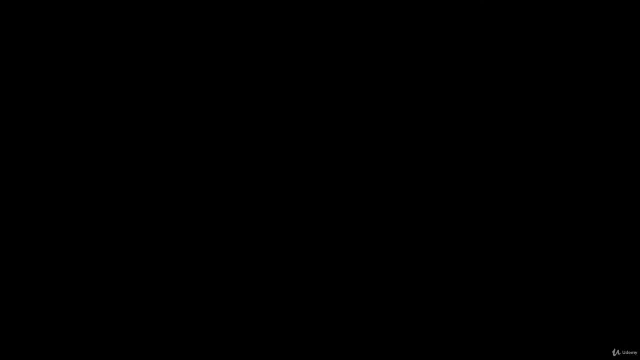 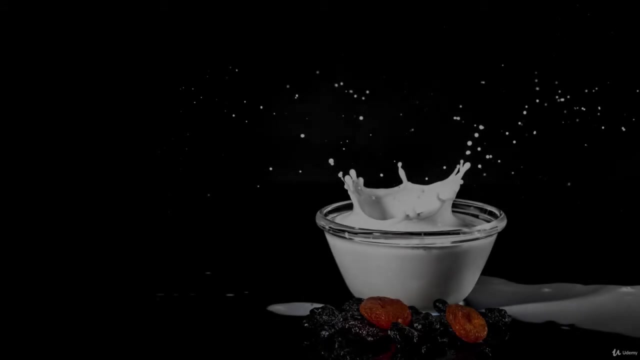 2000 and 4000 pixels across respectively. Though it's great to work with such high detail, it also makes for a larger file size. If you are working on, say, web design, large file size are usually not your friend. While the resolution tells us the pixel dimensions of an image, we can also know the pixel density. 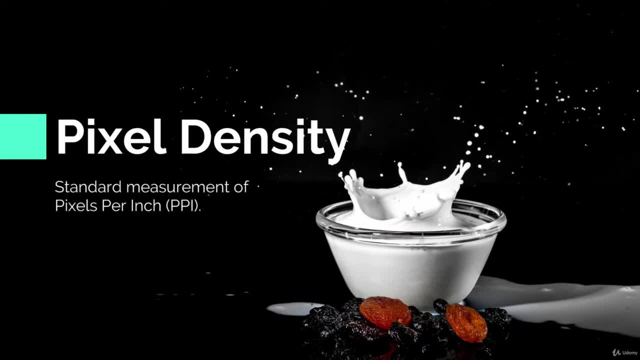 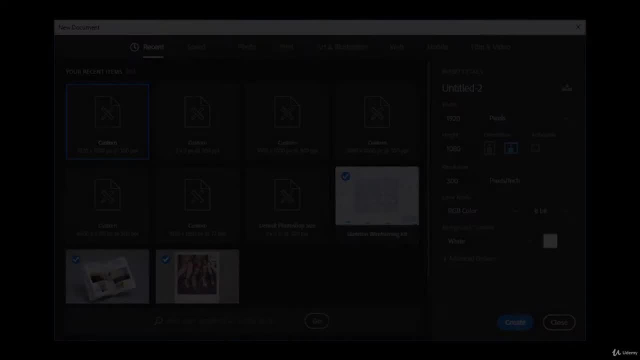 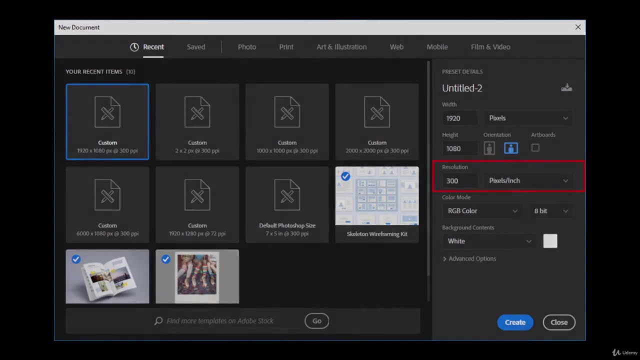 in what we call PPI or pixels per inch. You also might hear of pixels per centimeter if you are working in metric. This is the number used to say how densely compacted the pixels are to a certain size, like inches. Remember our 10x10 example. 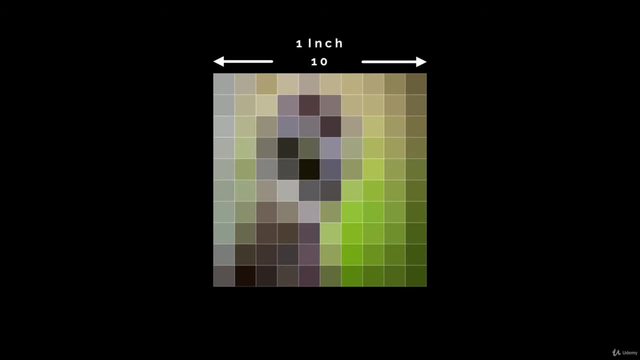 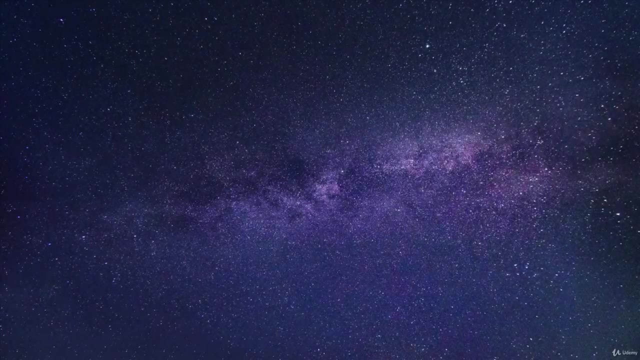 If that image was 1 inch, in both directions, we would say it has a 10 PPI density. If that image was 2 inches, then it would have a 5 PPI density. The more pixels per inch you have for your image, the smoother the image will look because of the density of the pixels. 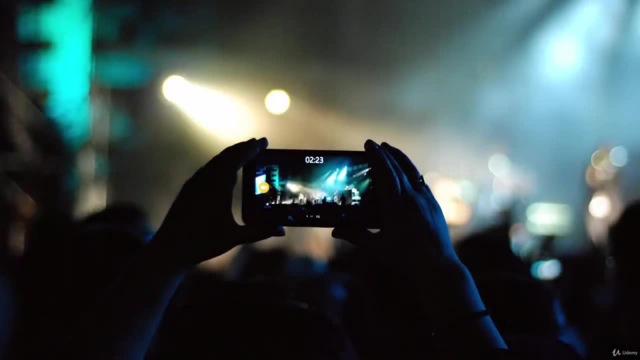 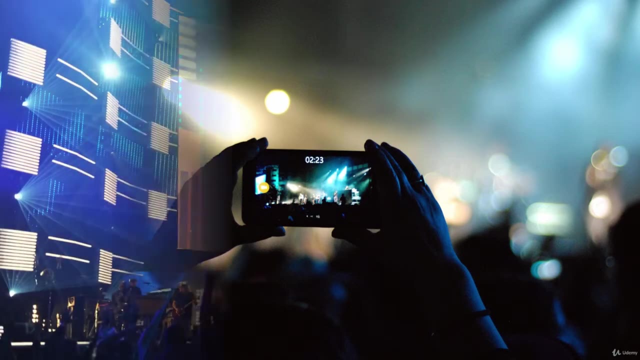 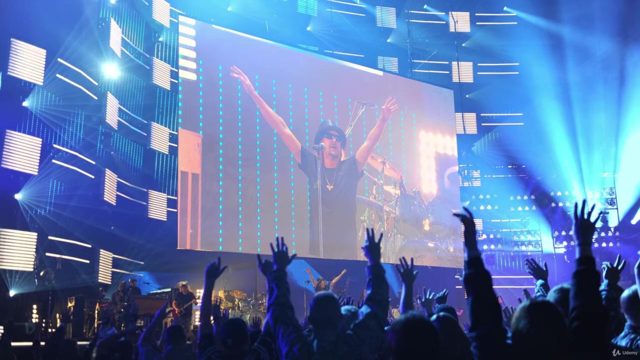 1920x1080 looks great on a smartphone because the pixels are tightly compacted into a smaller space and gives a higher resolution looking image, Whereas 1920x1080 can begin to look pixelated on a larger screen and a higher resolution needs to be used. 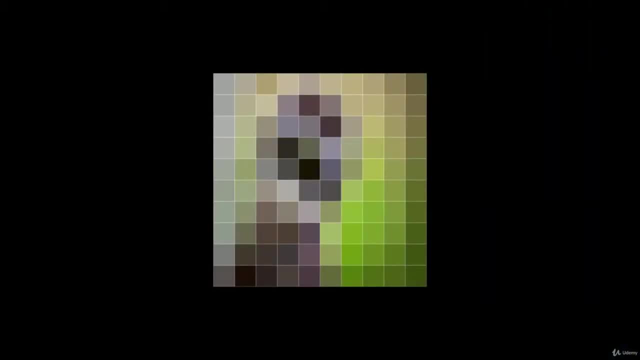 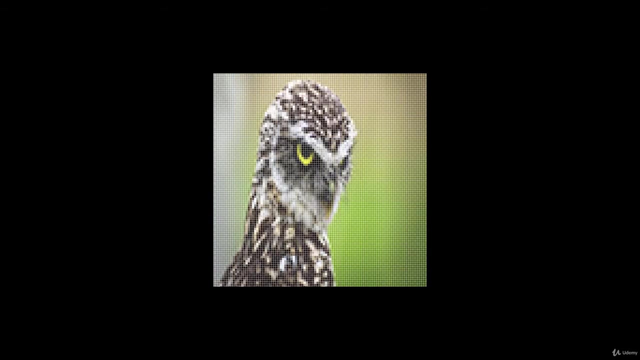 As you begin working with color, you will want to keep this information in mind, because the amount of pixels will determine the amount of available colors you can use. If you are working on a smaller resolution, you have a limit of the color choices available to you. As the resolution increases, you can blend a multitude of colors to get the 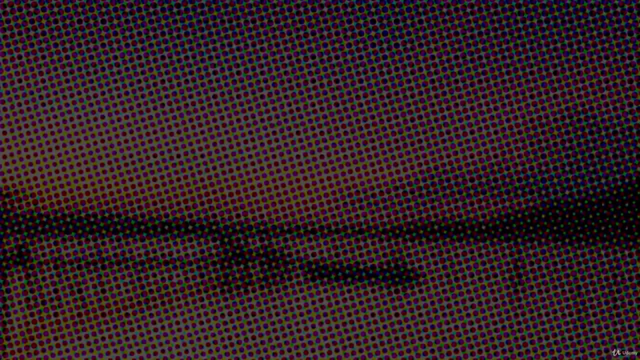 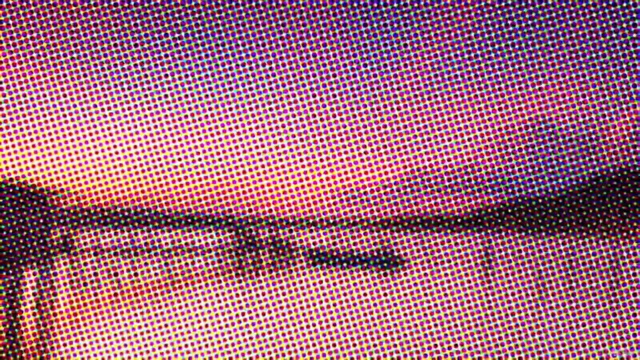 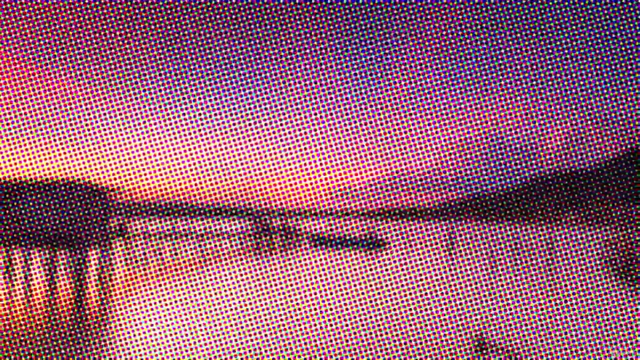 image. This is also exactly how print media works, only it's generally called DPI or dots per inch. That means how many dots of pigment will be laid down per inch for your image. Typically, you will want to have a very smooth image for print, and file size isn't such a big factor In that case you. 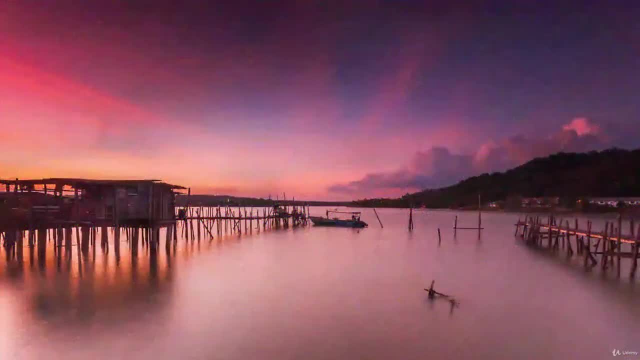 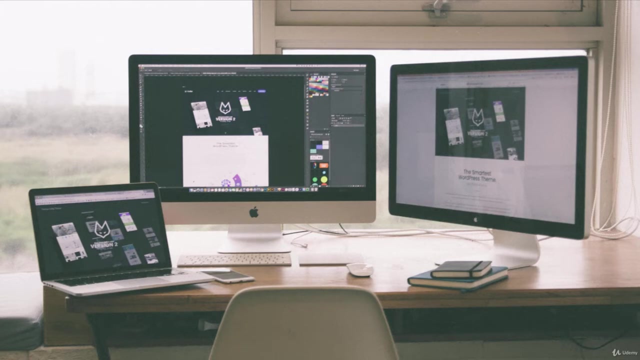 will use a higher resolution, like 300 dots per inch or more. That guarantees that you have a lot of pixels per inch of your design and get the best quality image possible. On the other hand, you generally want the lowest file size available without sacrificing. 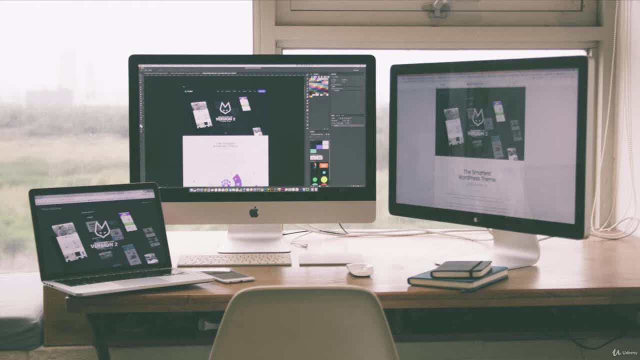 quality when you do web design work. That is because websites tend to have a lot of pixels per inch. That's why you should have a higher resolution. If you have a lot of pixels per inch, you will want to have a lower resolution. 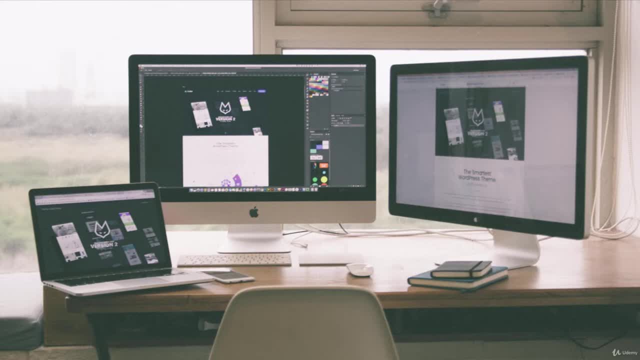 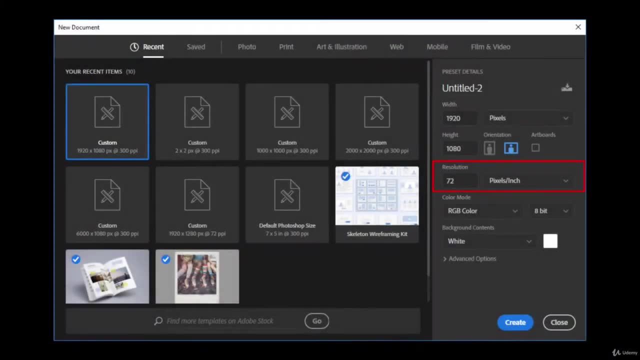 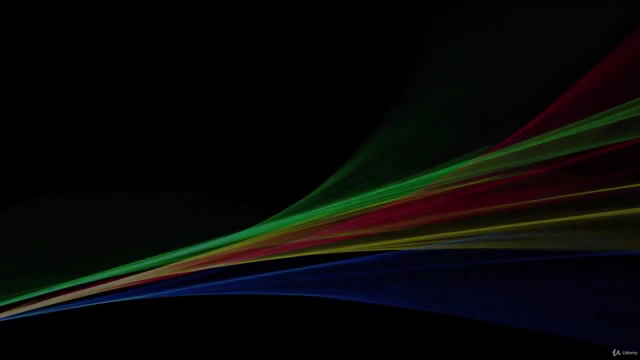 The lower the file size, the faster the website can load. The typical image resolution for web design work is 72 dots per inch, or pixels per inch, though that number can be changed to suit your needs. The final property you will want to look at is bit depth. Bit depth refers to the amount. 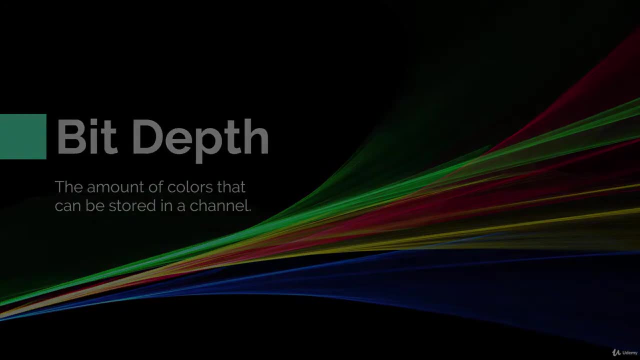 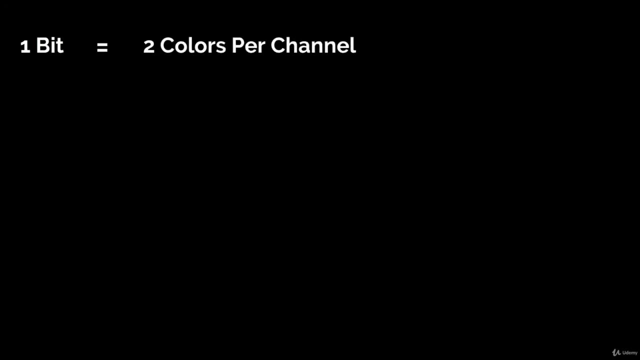 of colors that can be stored in any given image. In an image, one bit means that you will only receive two colors: black and white. Two bits gives you four colors. three bits gives you eight colors. four bits gives you 16 colors, and on up. 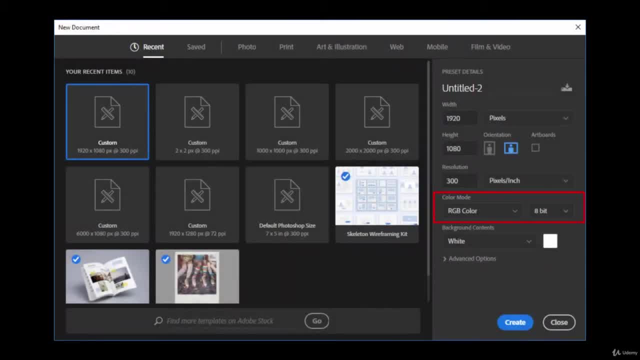 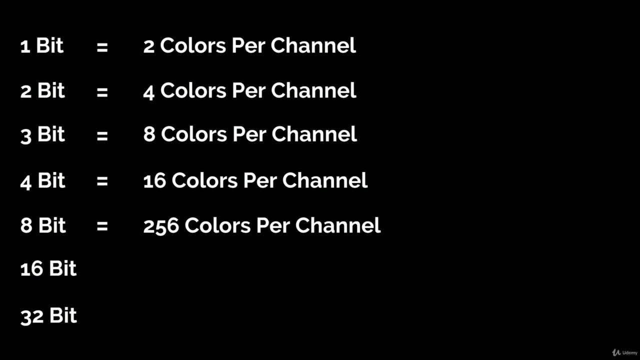 Typically you will use 8,, 16, or 32 bit depths. Eight bit depth is 256 colors and good for web design work. 8 bit depth is 256 colors and good for web design work. 16 bit depth is 65,536 colors and great for print work.